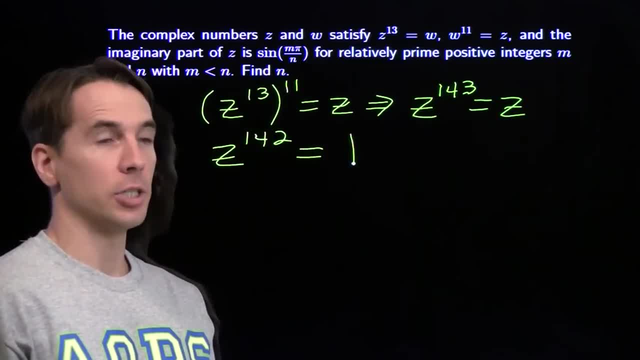 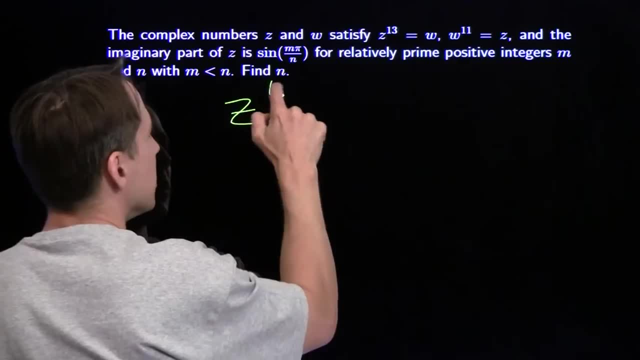 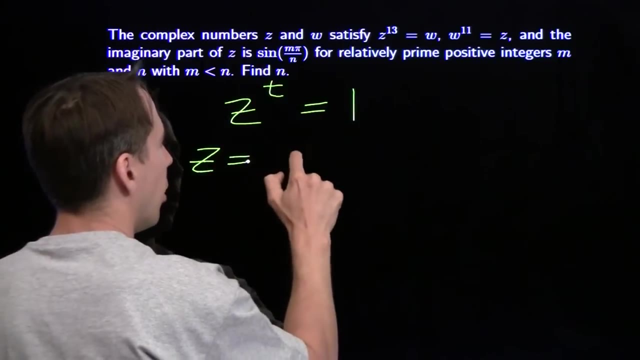 and if you don't know all about the roots of unity, then you're stuck. Now, quick, quick run through the roots of unity. Whenever we have an equation of this form- z to the t equals one where t is a positive integer, then the solutions are of: 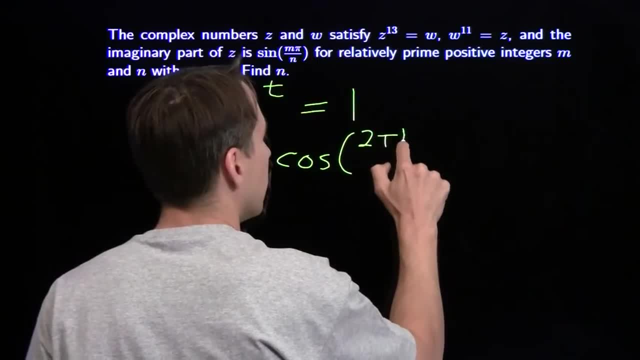 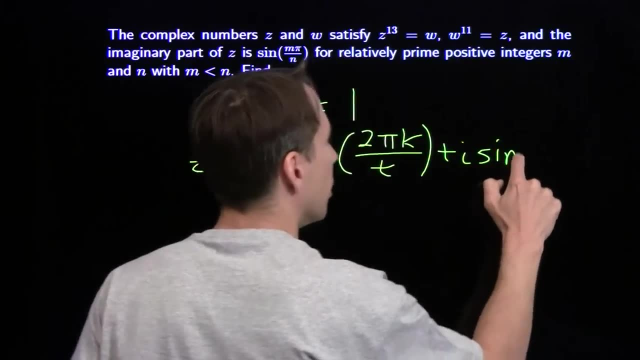 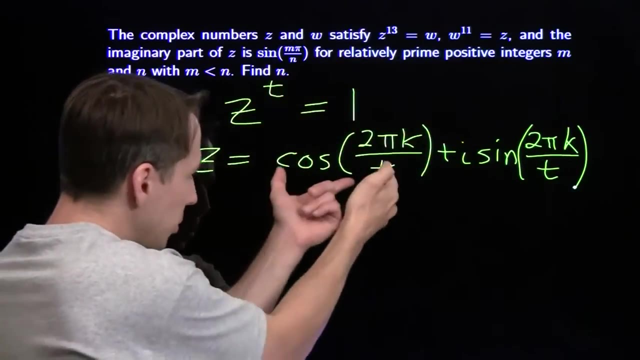 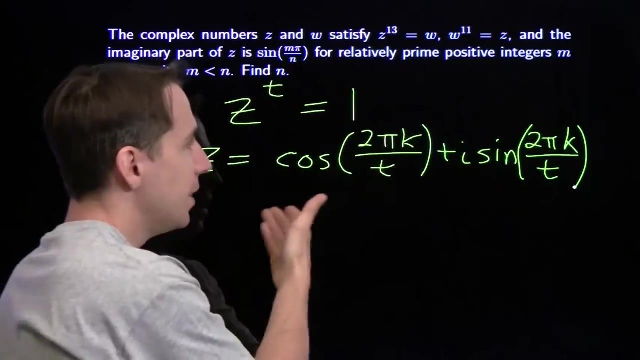 this form. All the solutions are generated by starting with this mess right here and then this one Where we take that power t, we stick it right there and then k is an integer. So we run k from zero up to t minus one and that'll give us all the t solutions, the t-th roots. 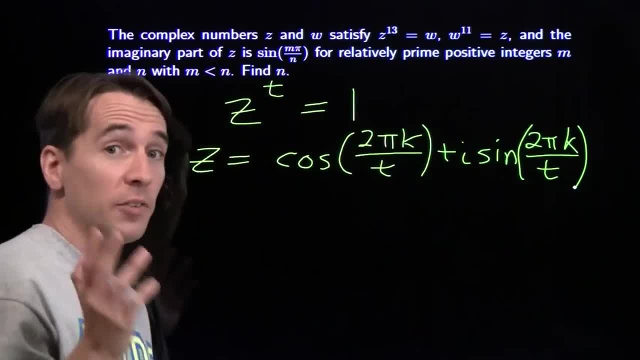 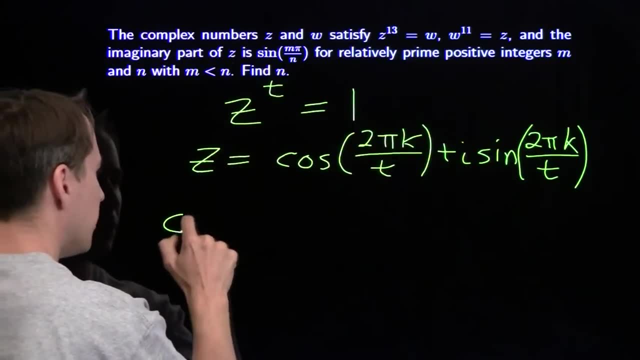 of unity to this equation. Now, the reason this is true is, if you happen to know DeMoivre's theorem, no matter how that's pronounced, this is a direct result of DeMoivre's theorem. And what DeMoivre's theorem tells us is, if we have cosine alpha plus i times sine alpha. 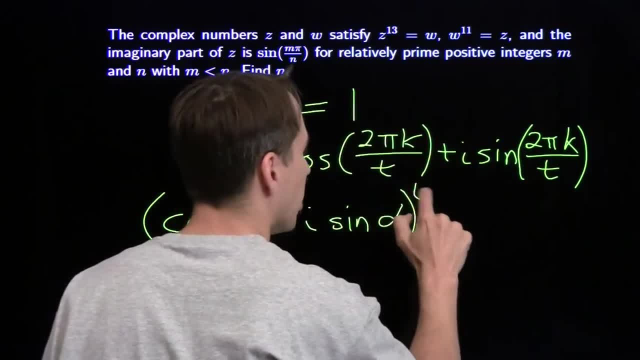 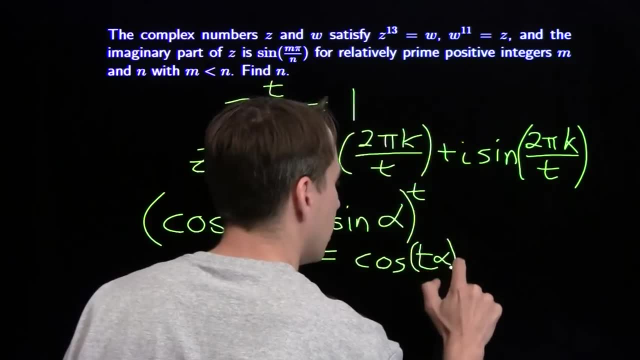 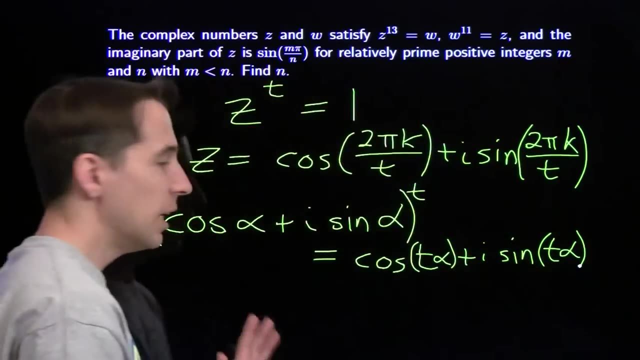 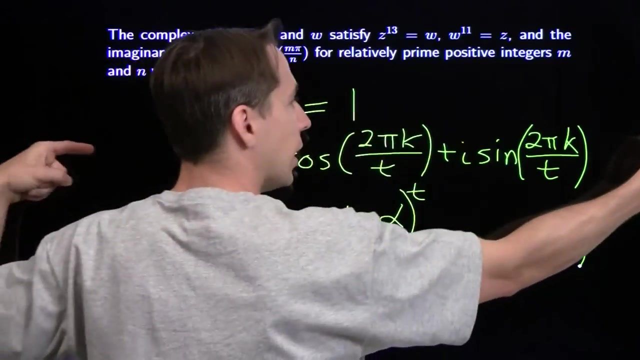 and we raise that up to some positive integer power, we get cosine t alpha plus i times sine t alpha. Now, if you've never seen DeMoivre's theorem before, see if you can start with this fact and figure out why the solutions to this equation look like this. And if you know some trig. 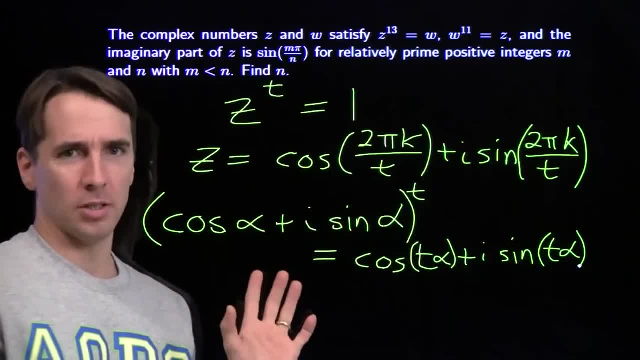 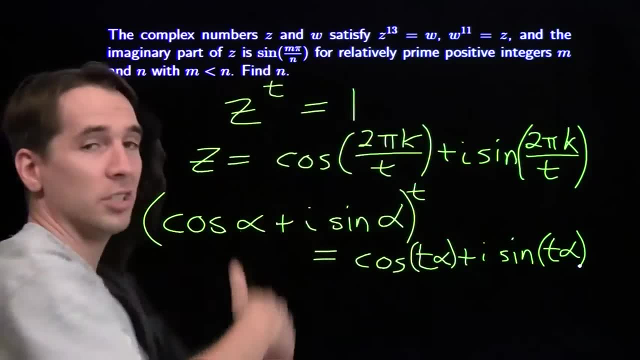 and have never seen DeMoivre's theorem before, then why don't you try to print out some of these and try proving this on your own? Start with t equals two and see what happens. and try t equals three and go from there. But like I said, if you didn't already know this, 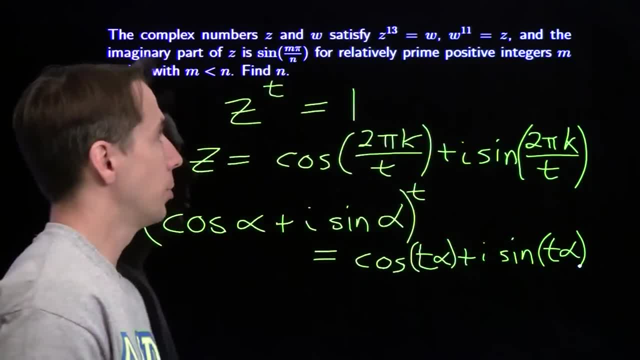 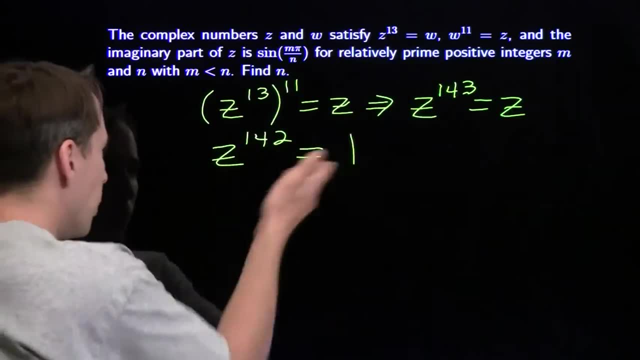 stuff coming into this problem. there is no way you're going to discover it during the problem, unless you're way, way smarter than I am, And that might be true. So now back to our story. Here's where we were. We have z to the 142nd equals 1, and. 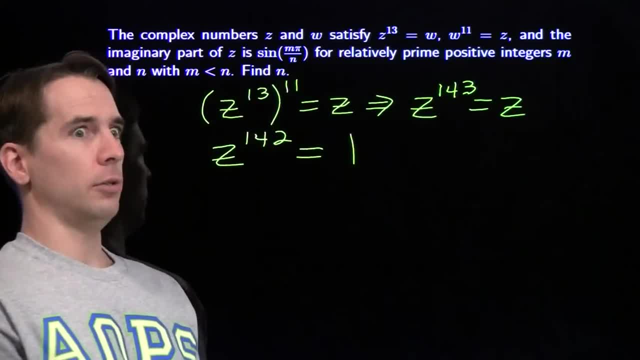 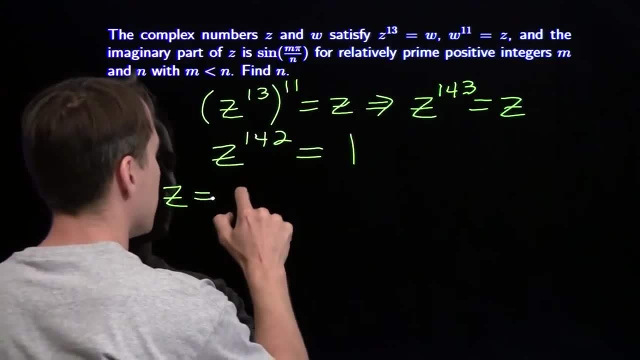 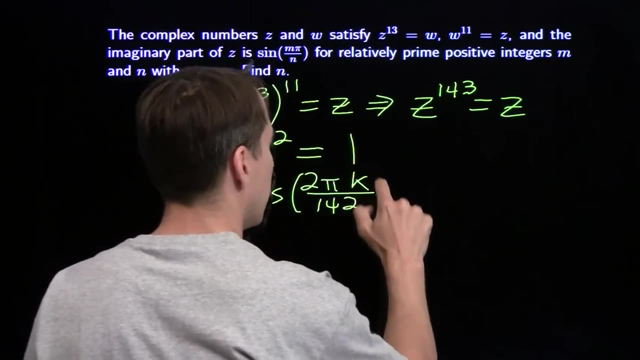 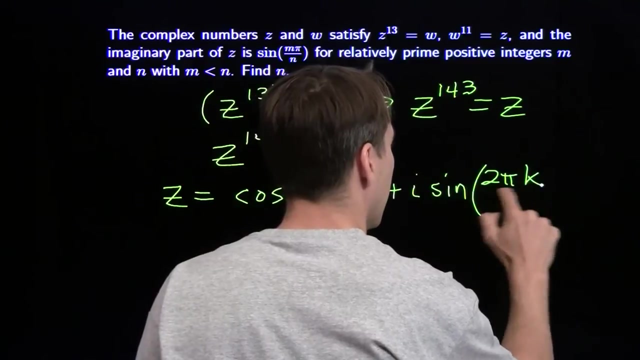 that tells us that the solutions are the 142,, 142nd roots of unity. Try saying that fast. And now we know what those look like. They look like this Cosine of 2 pi k over 142, plus i sine 2 pi k over 142.. All right,